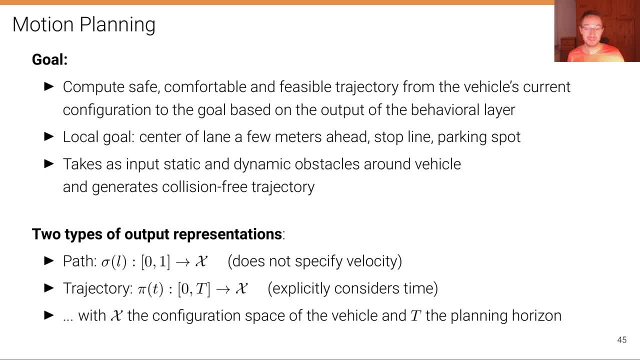 In other words, the trajectory output representation explicitly considers time. It explicitly asks our controller to move or steer the vehicle such that at any time specified here, as in the example, if there is an argument to that function, we are close to the corresponding configuration that's predicted by that function. 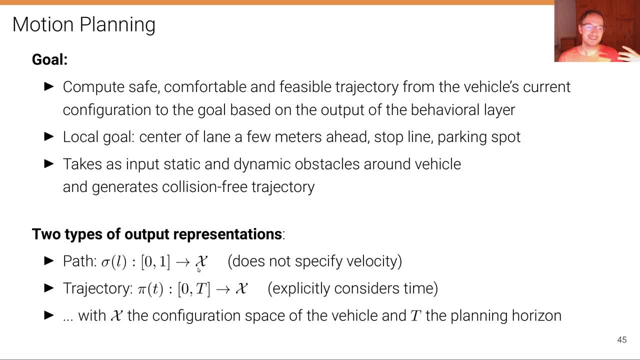 Well, in the case of a path, the controller itself must provide the logic for specifying the correct velocity. So in this case, here capital T is called the planning horizon and calligraphic x is the configuration space of the vehicle, For example the location of the vehicle and the heading of the vehicle in the simplest case, 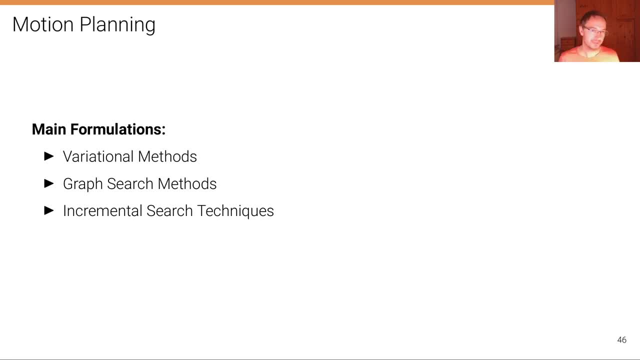 There's three dominating formulations for solving the motion planning problem. The first type of methods: use our variational methods, use variational inference techniques. Then there's graph search methods and incremental search techniques, And we'll have a brief look at that in a moment. 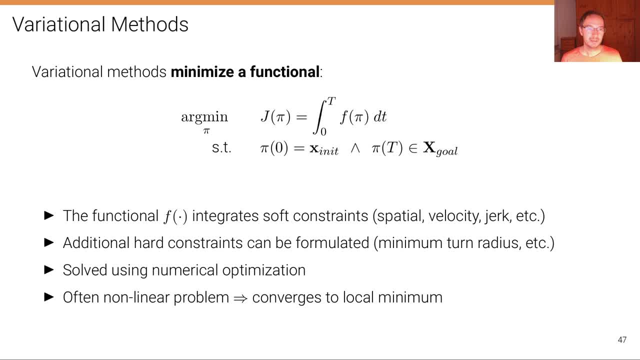 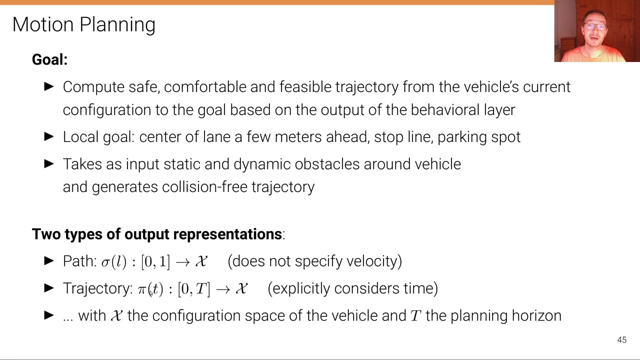 But not for now, Just to give you a brief look at all three of them. Variational methods, as you might know them from math, minimize a functional. So here we are trying to minimize that functional J. that itself depends on the functional F of Pi. 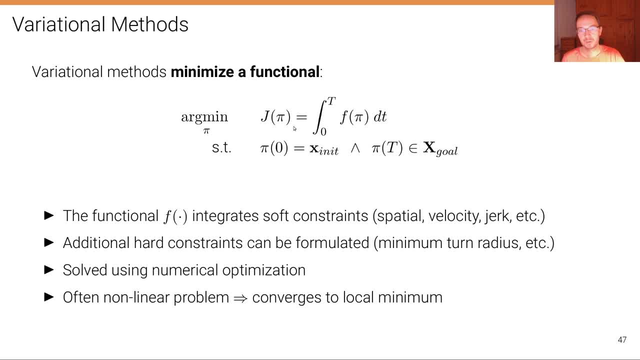 where the minimum function of a function- so we're minimizing that integral from zero to time horizon- t of that functional f of pi, where f integrates soft constraints such as constraints about the spatial location or the velocity or jerk that might be applied. but there's also additional hard constraints that can be formulated, such as the minimum turn radius that 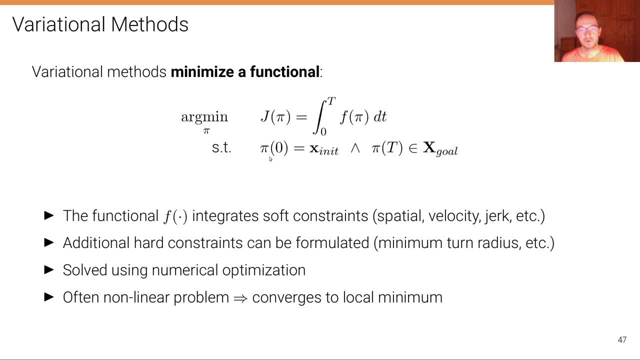 the vehicle can turn, or in this case, here also, of course, the starting location and the goal location, which, where the starting location is the location or the configuration of the vehicle at time zero and the goal location is the configuration of the vehicle at time capital t. this problem is then solved using standard numerical optimization techniques. 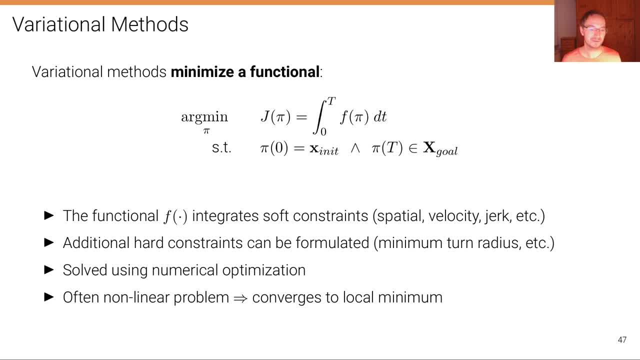 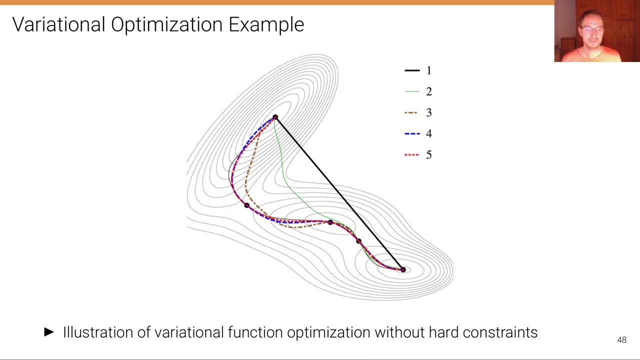 but in almost all cases this is a difficult, non-linear and non-convex optimization problem and therefore converges to a local minimum in order to avoid this. sometimes this optimization problem started from different initializations and other techniques are used in order to overcome this. so here's an illustration of a simple variational function optimization problem without any. 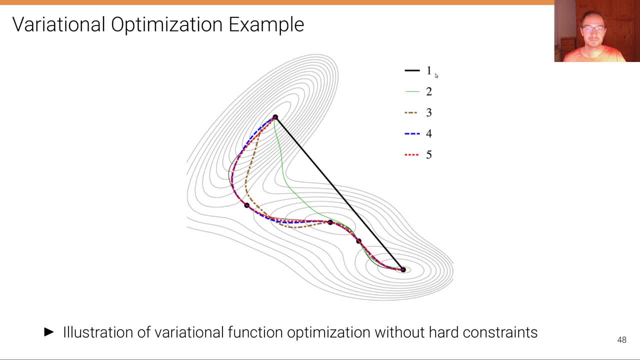 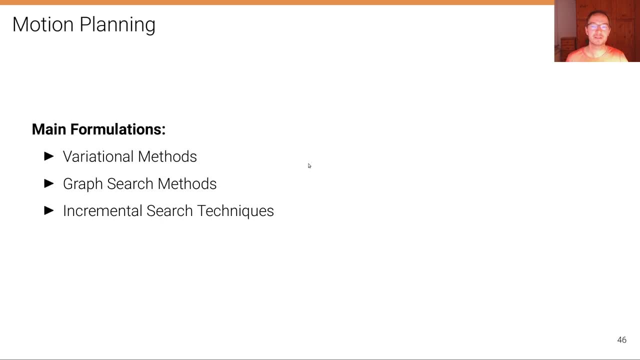 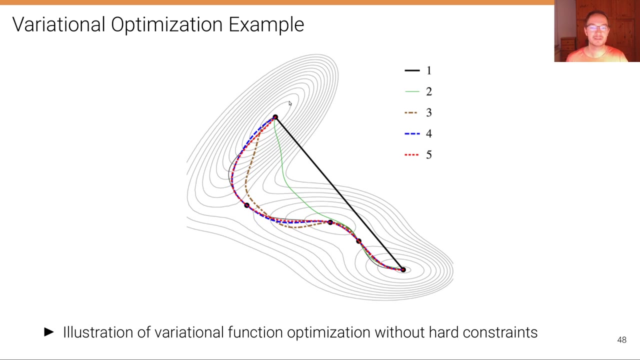 constraints. you can see the function here that's optimized. these are the different iterations here. in the background you can see the soft constraints that are integrated through this functional f, such as constraints on the spatial location, and you can see that over time this function here moves towards the minimum of this, this valley here. 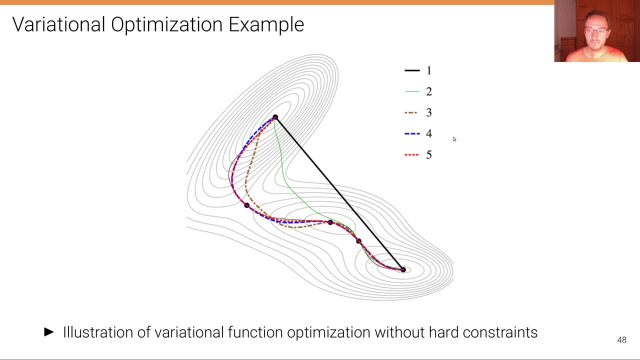 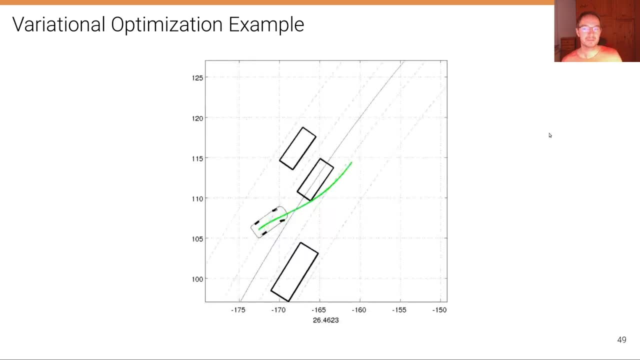 from the starting location to the goal location. the final iteration is the red one here. now let's look at a concrete example with a vehicle. this is a video i took from a former colleague, moritz welling, that worked intensively on these type of algorithms for 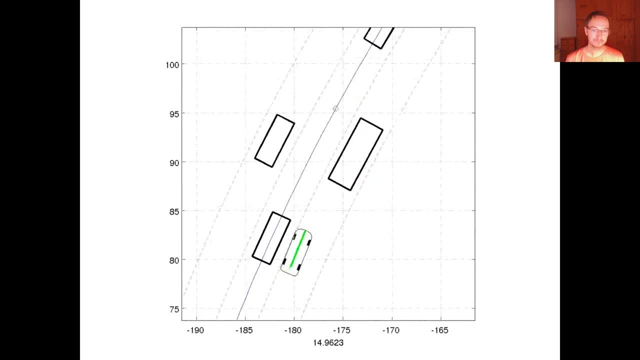 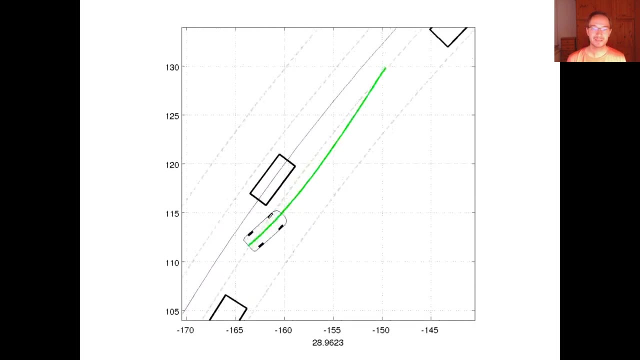 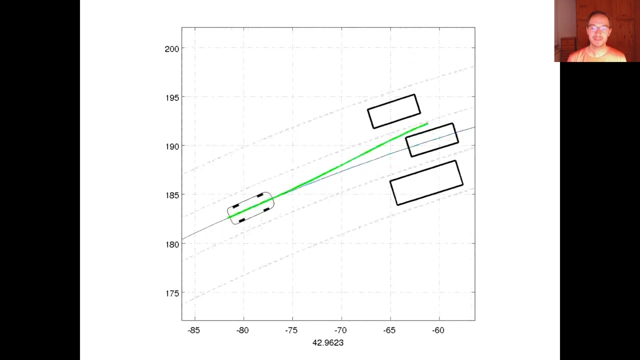 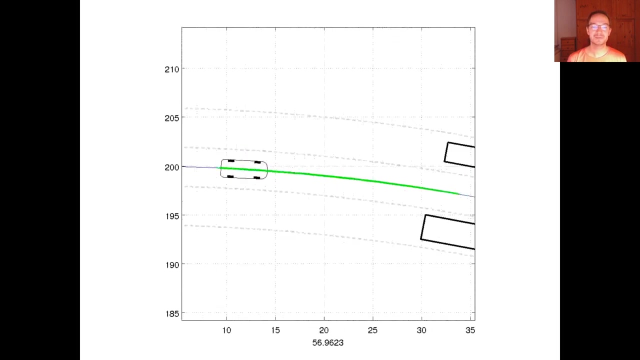 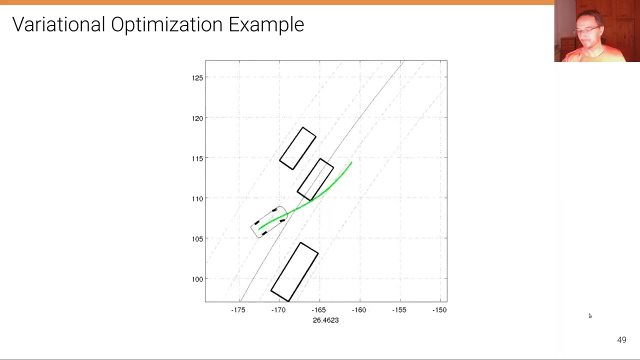 vehicle path planning and motion planning. you can see how this vehicle is well i i wouldn't recommend conducting these maneuvers in practice, but you can see how sophisticated that planner is and how, how accurately and aggressively it can actually be tuned to plan such trajectories. okay, an alternative to variational optimization. 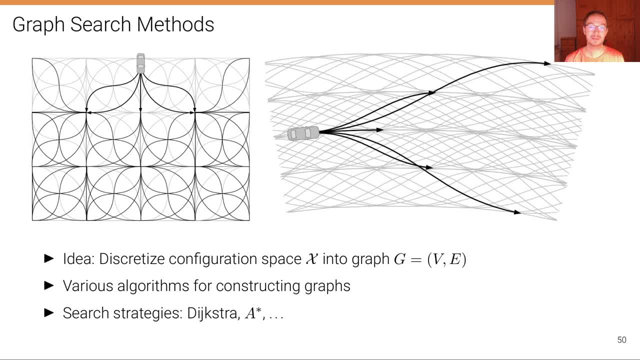 is to use graph search methods as the ones that we have discussed before, such as dixtra or a star, but in order to use them, we first have to discretize the configuration space x into a graph comprising vertices and edges as we've seen them before, and there's various algorithms in the 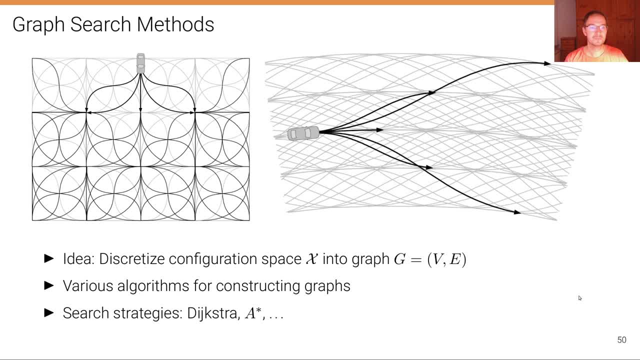 literature for constructing such graphs. here's a simple example for parking maneuvers on the left, where the configuration space is discretized based on this grid structure. here on the right you can see different lanes on the highway where lane change maneuvers are modeled based on a discretization of the configuration space. 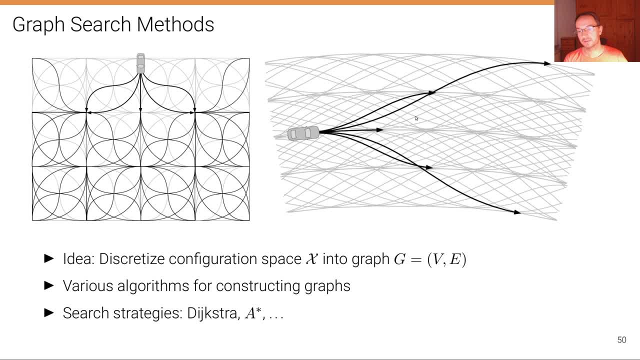 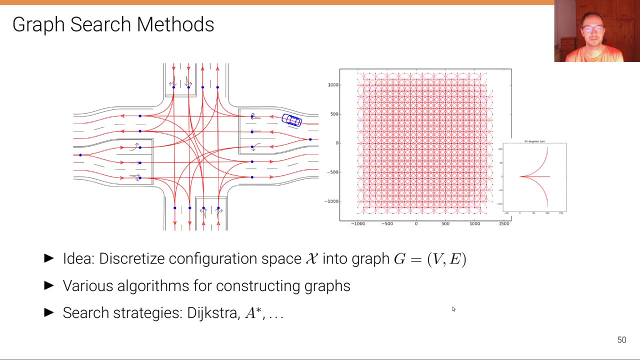 each of these gray and black trajectories are trajectories that can be taken by the vehicle, and so, through this discretization, we can now formulate it as a graph search problem. here's another example for intersection, where you can see how the different lanes and the different possible possibilities to 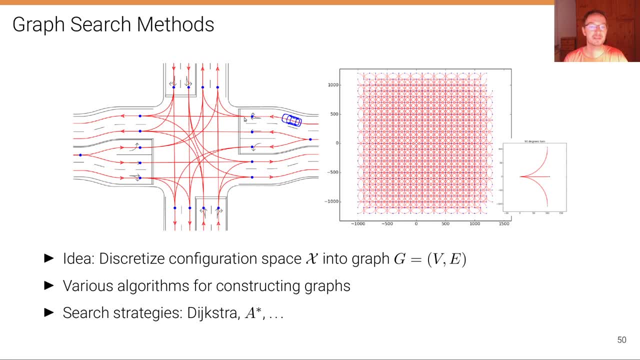 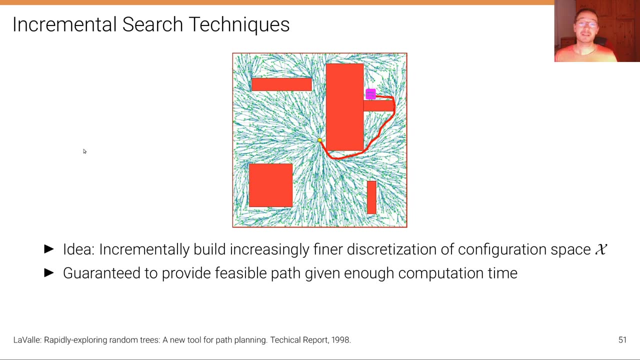 cross an intersection are discretized. so for example, this vehicle: here it can either go straight or it can go to the right, and if it goes to the right it can either move towards this lane here or towards this lane. and finally, there's also incremental search techniques. 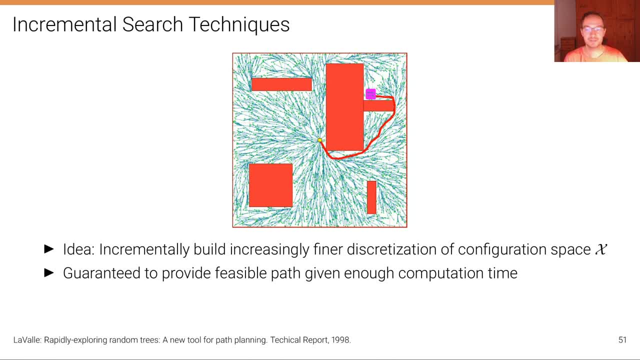 where the idea is to incrementally build increasingly finer discretization of the configuration space x, which are guaranteed to provide a feasible path given enough computation time. however, the computation time can be unbounded, and the prominent example of such algorithms here is the so-called rapidly exploring random trees algorithm. 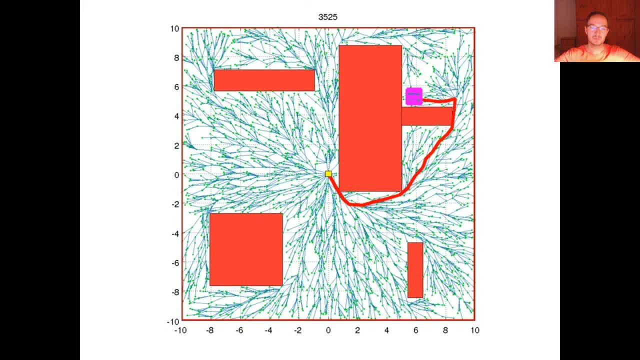 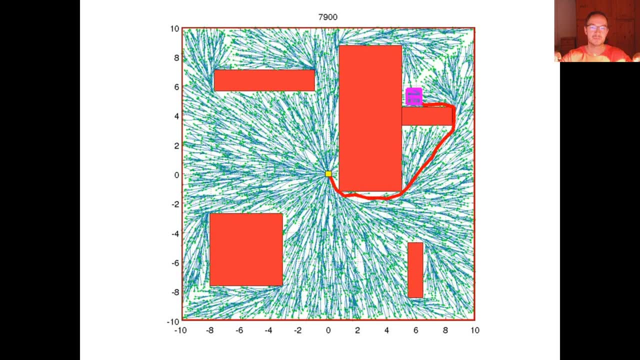 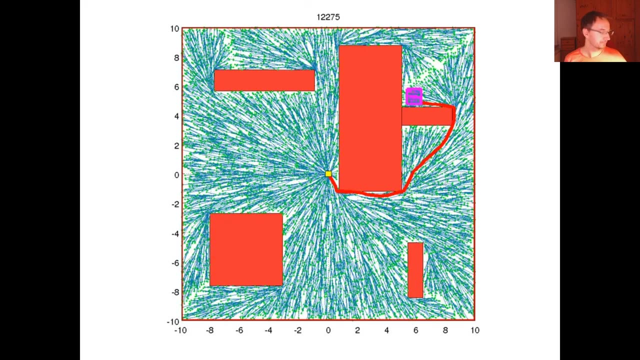 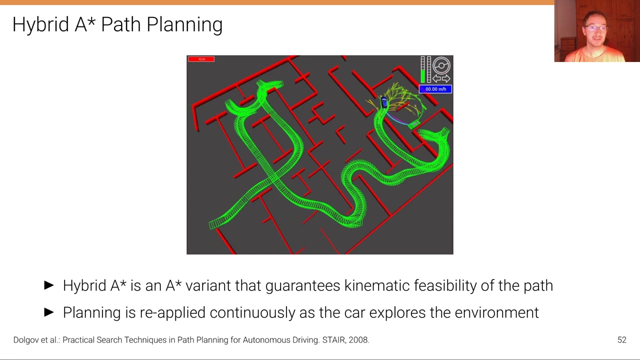 which is shown here. so in the beginning it randomly explores the space and finds the course path to the goal, and then it it much more densely samples the space in order to refine that path and make it better. and here's another example for the for a planning scenario with the a star algorithm. 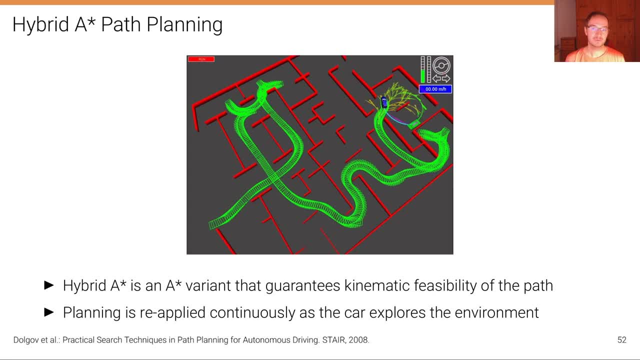 this is actually, um, an example from the stanley vehicle, where they used what they call the hybrid, a star algorithm, which is an a star variant that guarantees kinematic feasibility of the path, where planning is reapplied continuously as the car explores the environment. now here's an actual result of applying this a style with them for a vehicle. 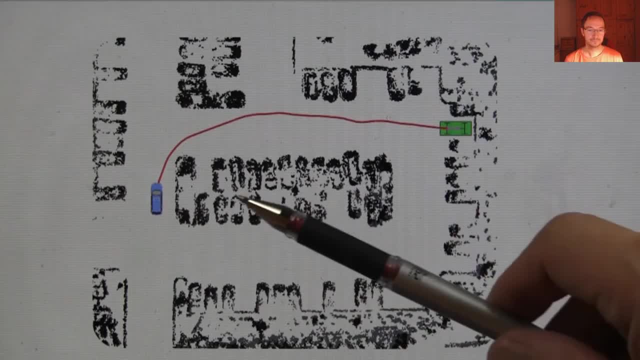 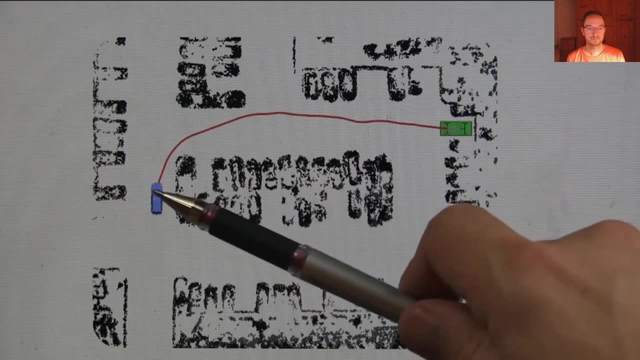 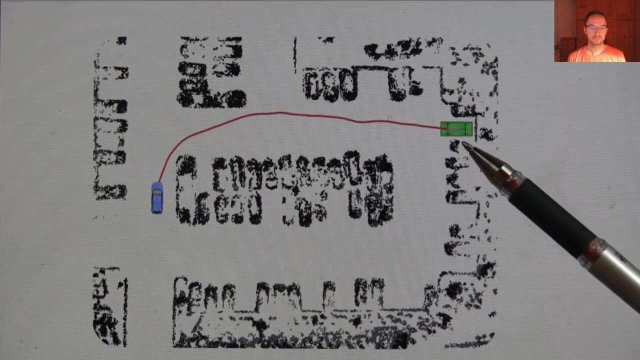 that sits over here. real obstacles: these are laser scans of parked cars and a target location over here and where the curve isn't super smooth, you can still see it is a very smooth curve. it is able to find a continuous and drivable curve to the parking location over here. 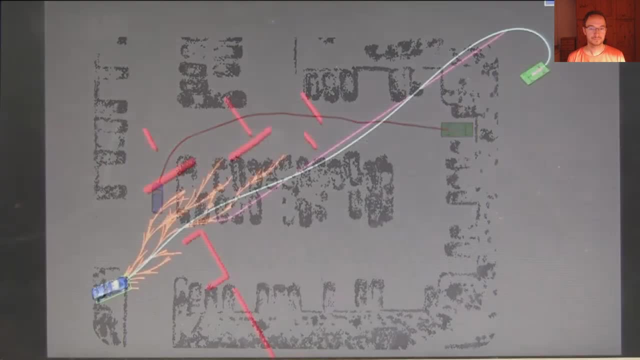 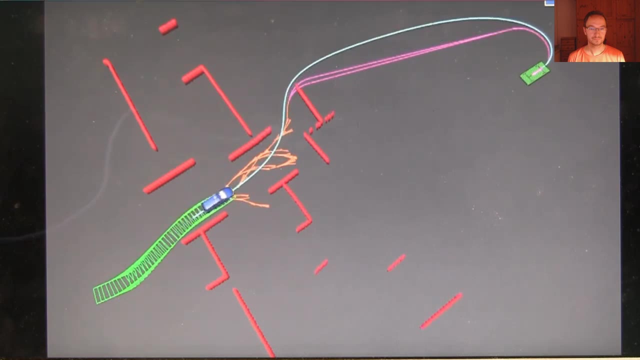 by this small but important modification of a star. now there's a few other modifications of a star which i can't go into detail, but here you can see a typical attempt of a robot to navigate a parking lot. here in simulation you can see the tree that is being expanded in that search. 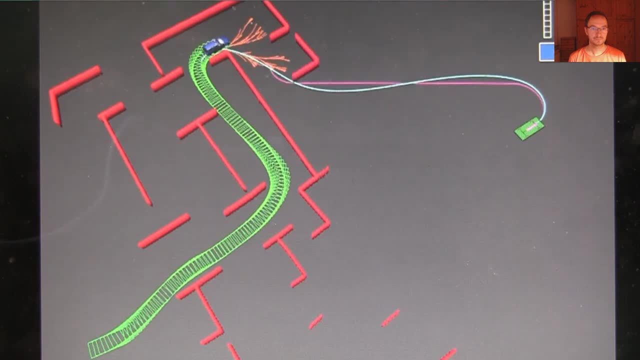 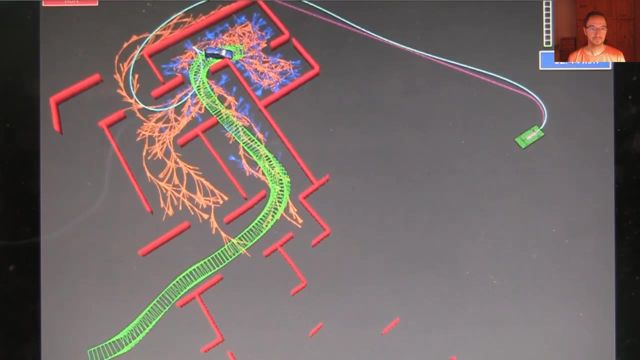 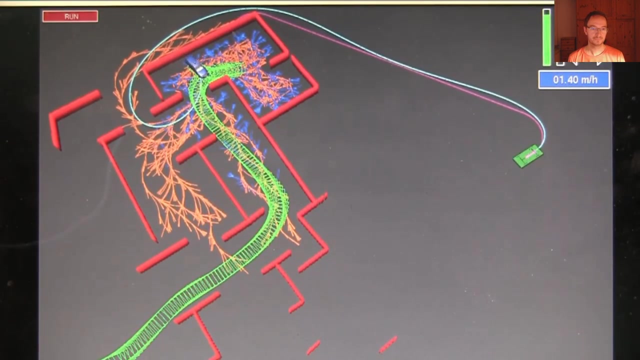 and every time it gets stuck it does a new way. you can see how the map is being acquired as the robot moves. in its state description of the robot, it not only considers the x, y and heading direction, but also allows over to go forward and backwards. and driving backwards is a different state than going forwards. and now you can see how it backs up. 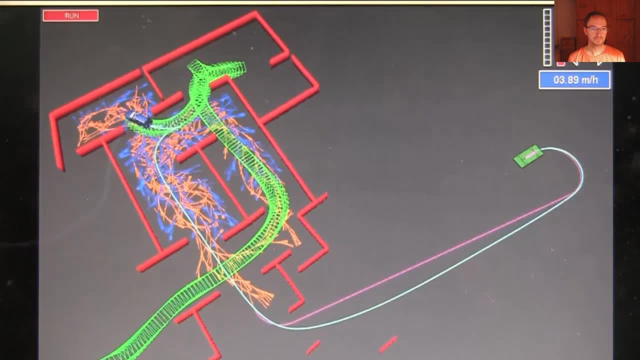 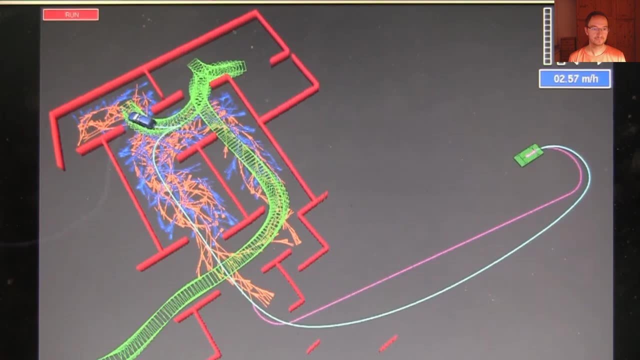 finds a new path in this incomplete maze until it finally is able to reach the goal location through an actual opening. it's uh, we made this maze really hard to take, so we're going to test our items. the nice thing is, these algorithms work in almost real time. 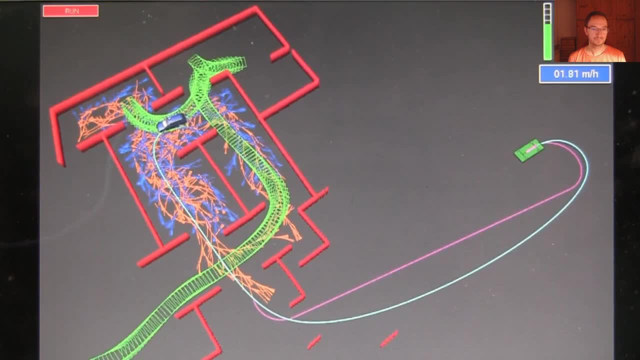 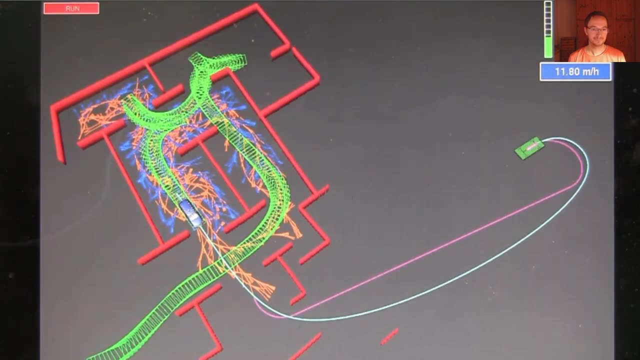 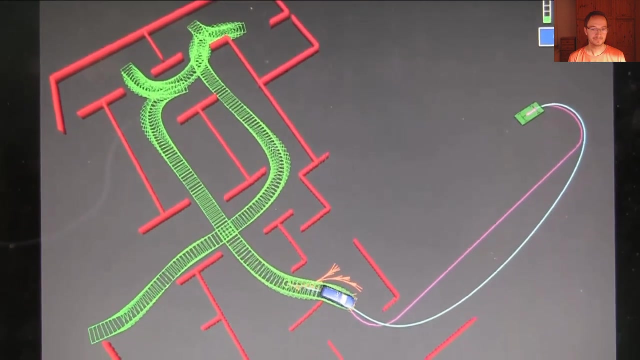 it takes less than a tenth of a second to build this entire search tree and the robot is able to navigate this parking lot really, really efficiently. this was one of the fastest motion planning algorithms that i saw in the DARPA urban challenge, in fact, in all of robotics. 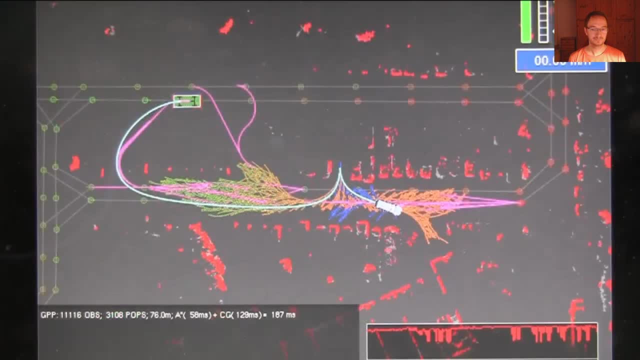 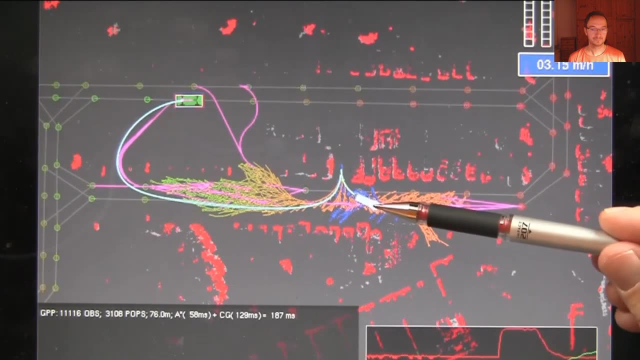 it's been one of the fastest algorithms i've personally seen in my life. and here is the same algorithm applied to an actual example, using our robot junior. it's driving over here, it wishes to get over there and you can see it back up into a parking gap over here. 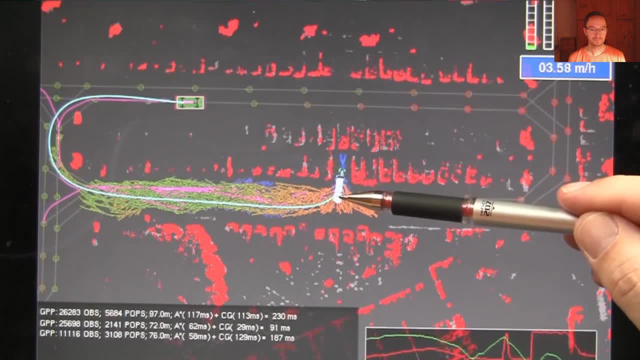 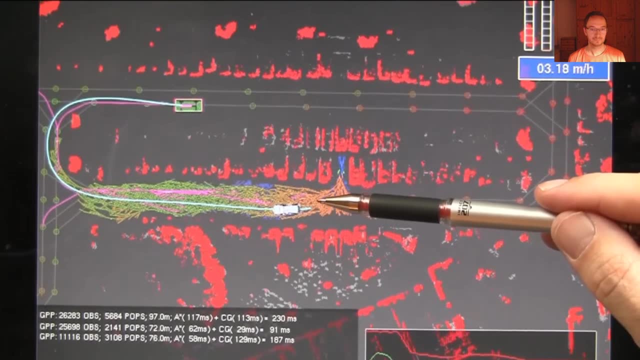 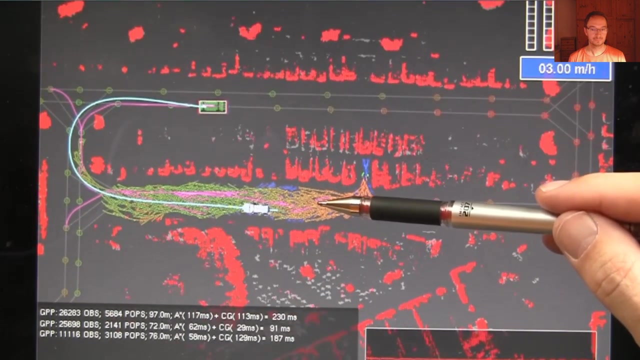 which is an amazing precision for a robot, and then move forward along the line over here. our state space is three, i guess four- dimensional. it comprises x, y, heading direction and whether the car is going forward and backward. there's a cost to changing direction, so it doesn't change. 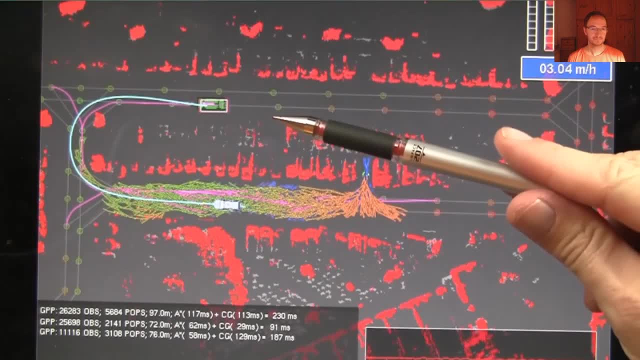 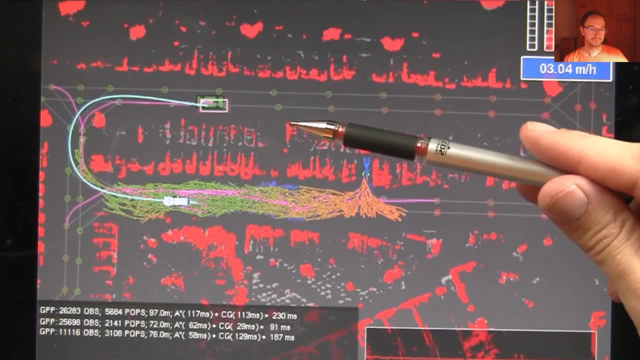 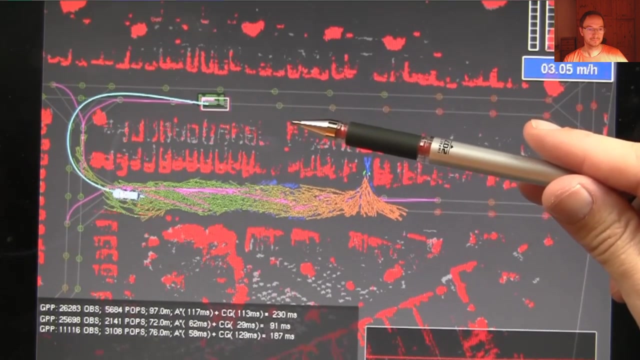 direction too often and you can see it navigate to its target location details i'm not telling you. include that the trajectory that the planner generates is subsequently smoothed using a quadratic smoother, so that we get rid of the kinks and the car drives much nicer as a result. 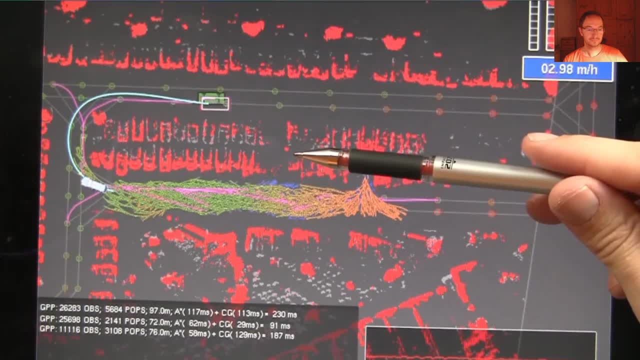 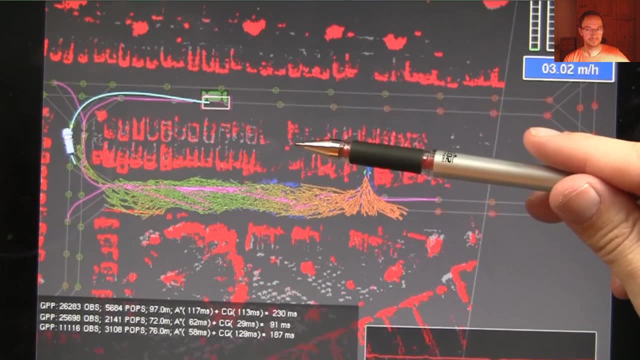 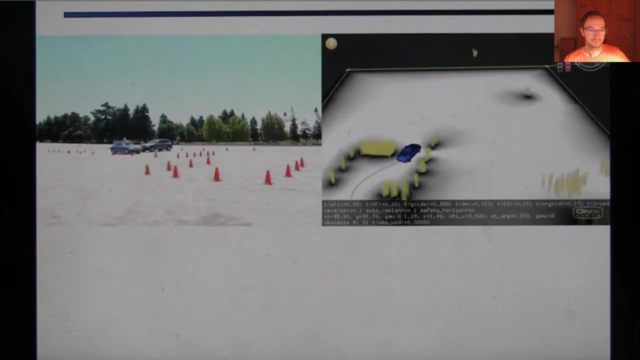 but the workhorse here that does all the work to find the best path is actually a star modified into hybrid. a star, as i told you, and in this final video we see the car navigating a parking lot with lots of traffic cones on the left. you see the video imagery. 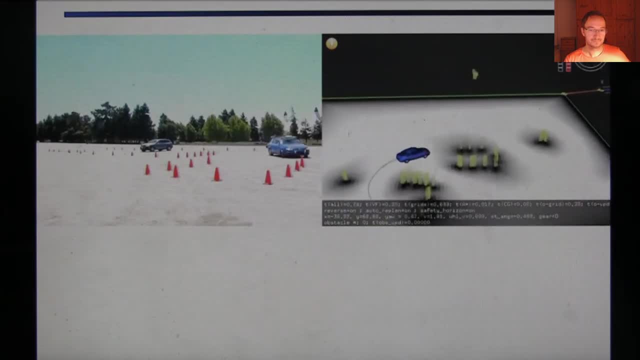 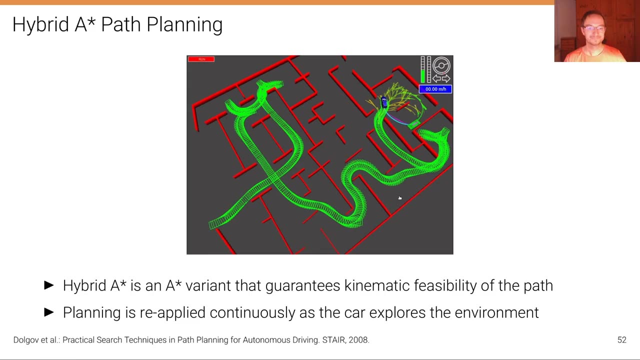 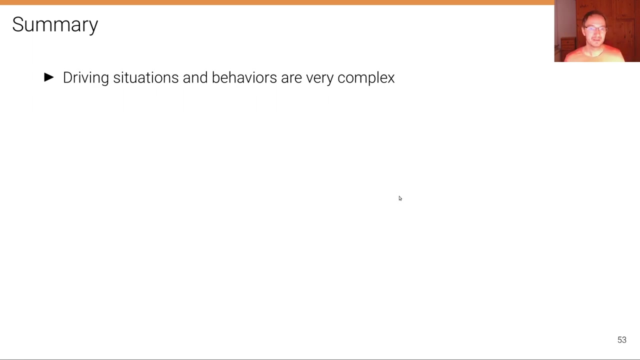 on the right side, you can see the internal map and the path planner, and it attempts to park itself in the designated spot on the left. now here's an okay, so that's all for today. let's summarize this lecture briefly. we've seen that driving situations and behaviors 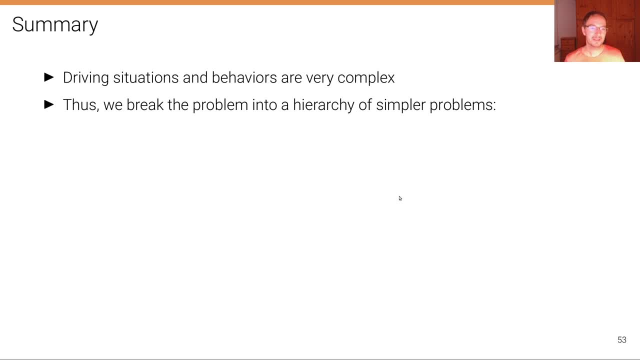 or can be very complex, and therefore it's a good idea to break down the problem into a hierarchy of simpler problems, such as route planning, behavior planning and motion planning. each of these problems is tailored to its scope and level of abstraction. road networks can be represented as weighted directed graphs, and we have seen that dykstra's algorithm finds the shortest path in 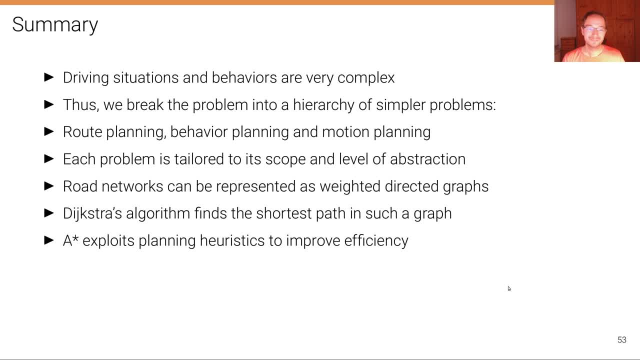 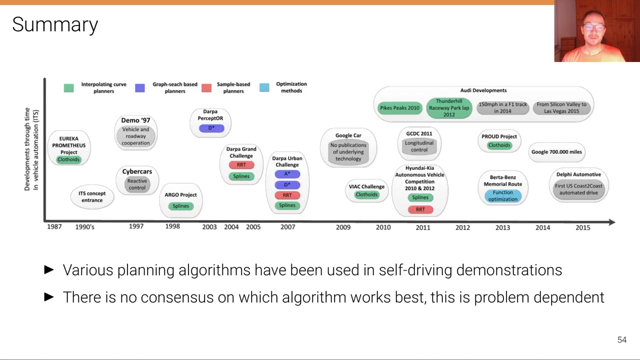 such a graph, however, a star is even more efficient and exploits planning heuristics to improve its efficiency. we've also seen that behavior planning can be implemented using finite state machines and for motion planning, variational and graph search methods are often used. various planning algorithms have been used in self-driving demonstrations, and here's a little.